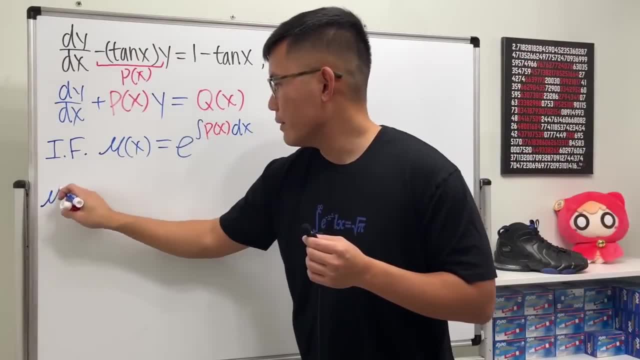 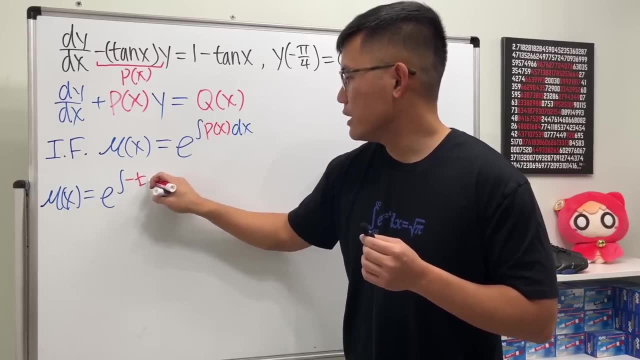 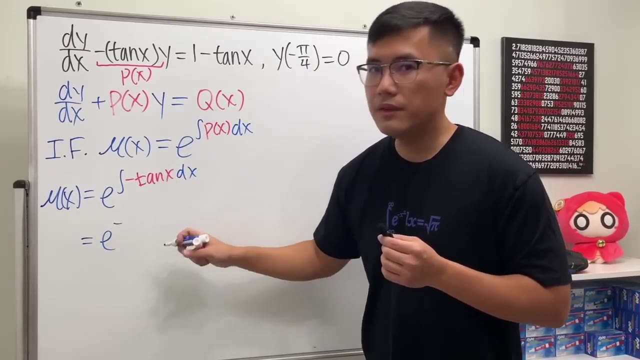 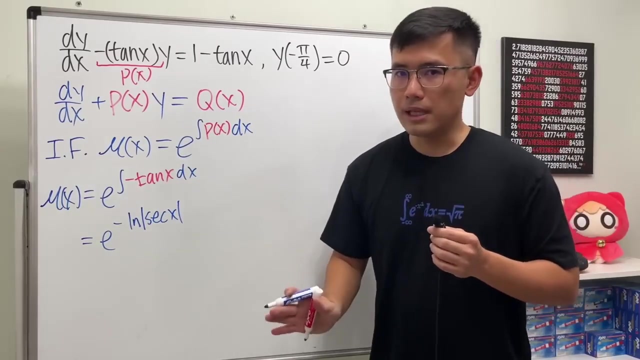 is negative tangent x. So when we have mu of x, we will have to do the integral here, and that's negative tangent x, dx. Well, this is just e and the negative is still negative. and the integral of tangent x is ln, absolute value of secant x. And you don't need a plus c here, because if you do, 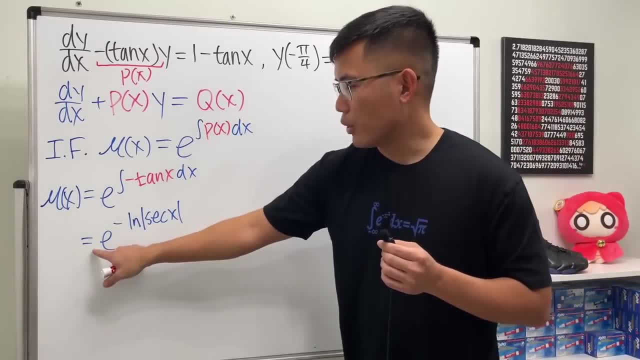 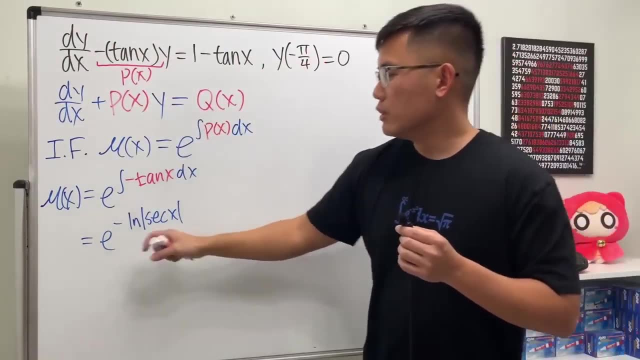 put a plus c, that becomes a coefficient. here And later on we'll multiply this integrating factor throughout this differential equation. So if you have like a, c or whatever here, later on you can divide everybody by that special constant. so it doesn't matter. 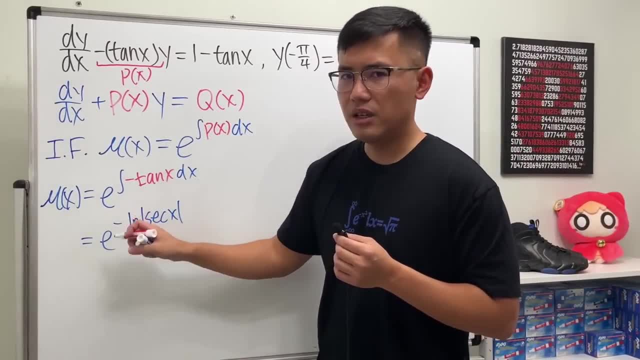 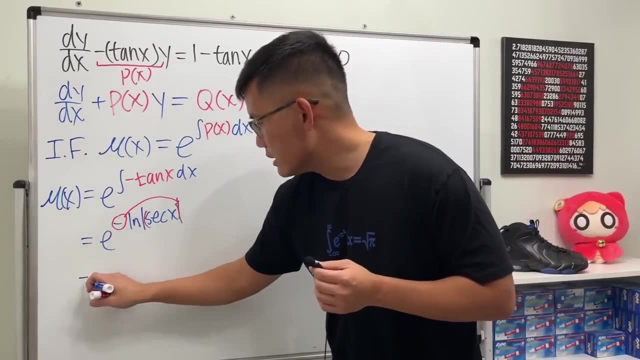 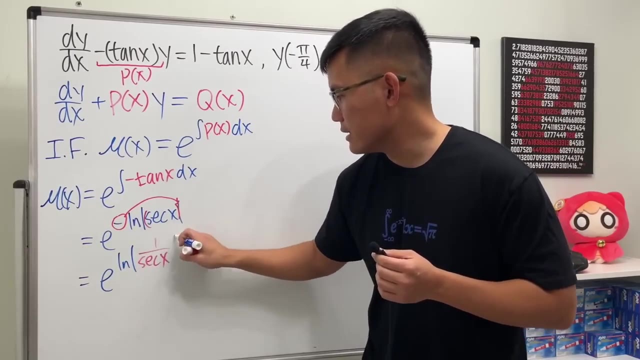 We can almost cancel out the e and ln, but we have a negative here spotting us. Let's put a negative to here. Becomes the negative 1 power. So this is e to the ln, absolute value of 1 over secant x like this. So 1 over this is not going to be the negative 1 here, as the inverse. all right. 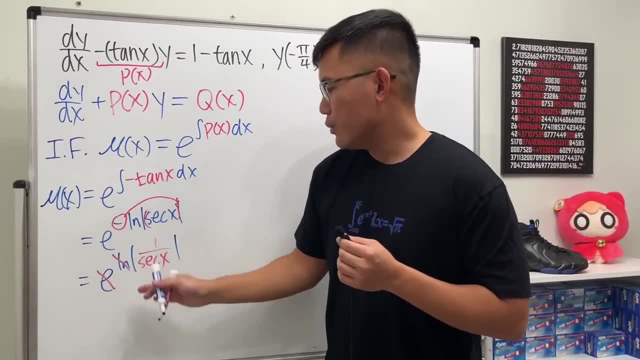 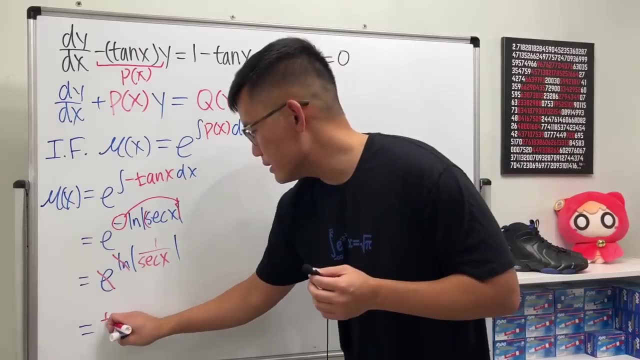 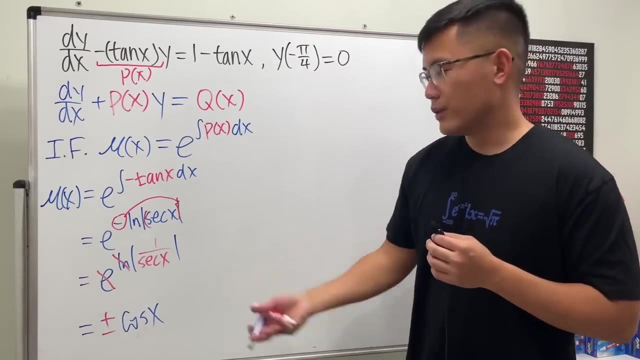 Now we can cancel out e and ln and we have this absolute value spotting us. Well, to take out the absolute value, of course we consider the plus or minus And of course 1 over secant x is the same as cosine x. What do we do? The positive version or the negative version doesn't matter. Imagine: 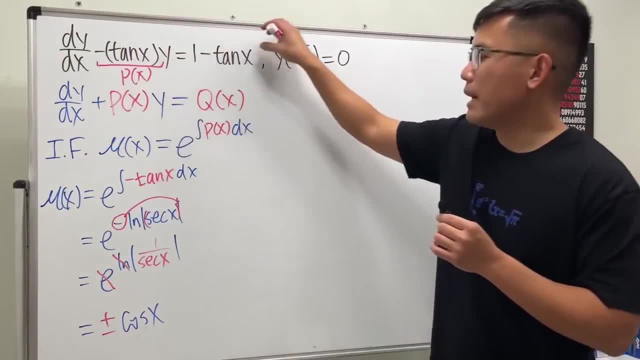 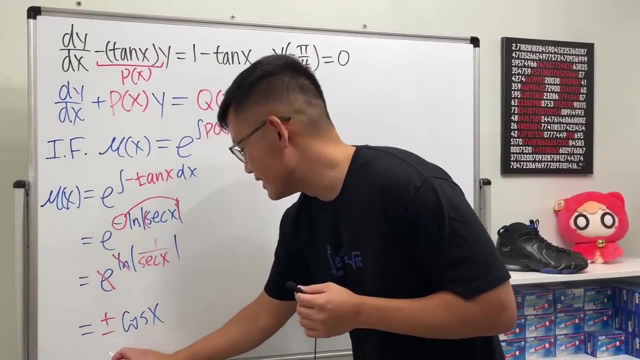 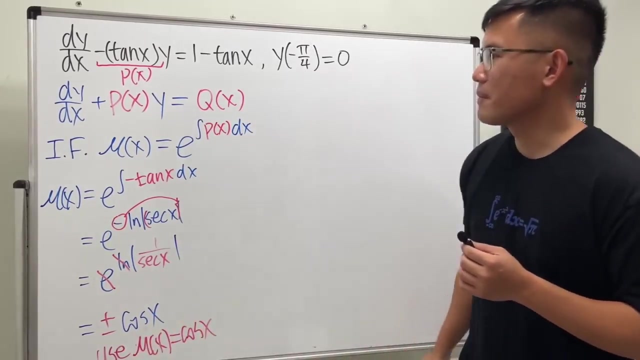 if you choose a negative cosine, you multiply everybody by negative cosine. Guess what? We can multiply everybody by negative. So let's not do that. so let's just use, let's just use mu of x for cosine x, just the positive version. So how it works is that we look at this original differential. 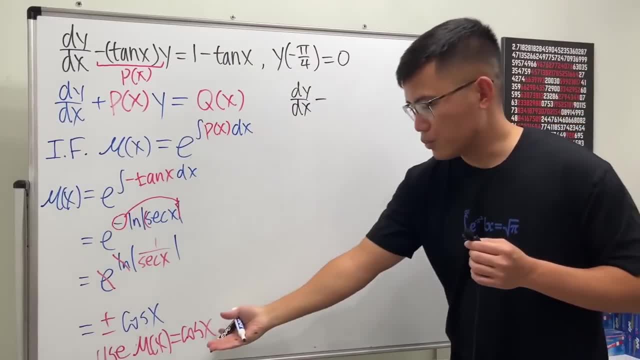 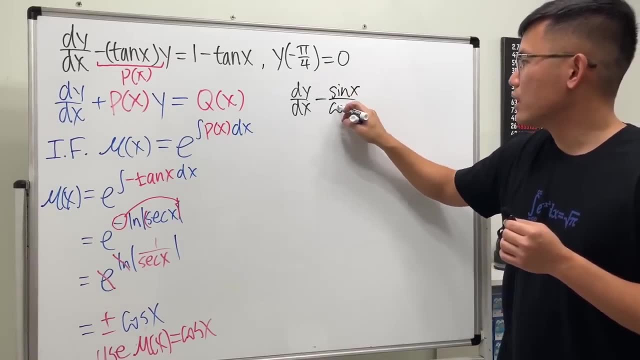 equation again Divided x minus for tangent, because we have to multiply by cosine. Let's go ahead and just write this: sine x over cosine x and then multiply it by我就 念 θ, performed by βM. So if you know what it would do if we do that and multiply anything by the physical visitor. then you can have truly infinite mu. So you canish over dX and you can change this: λ use for cosine Cyrus- inject this times xễ tray Salvador, Okay. So if this is dumplings, let me tell you this: we can really teach you not this combo. So if you 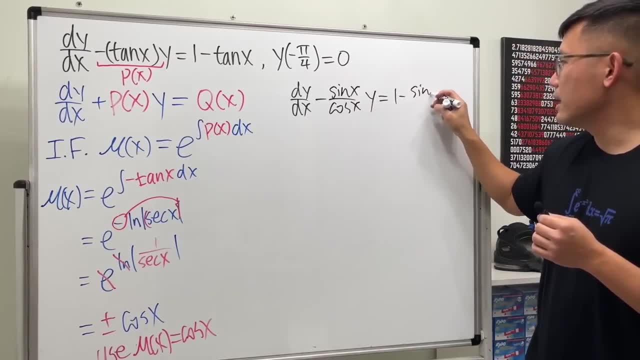 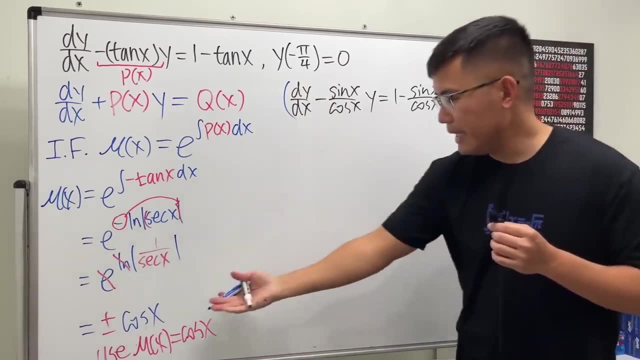 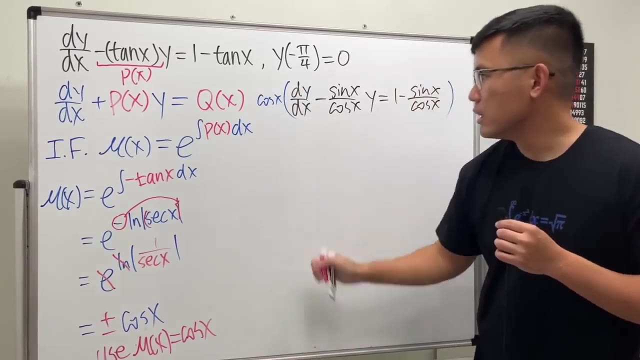 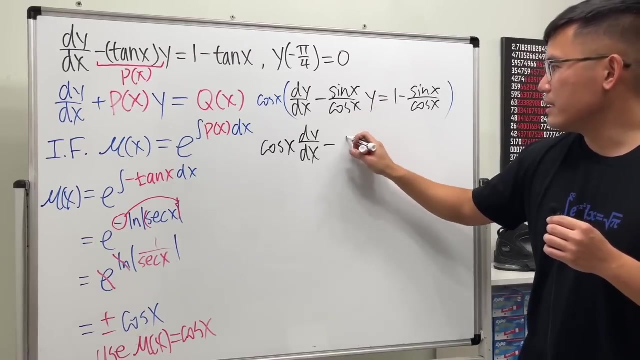 by y, that's equal to 1 minus. again, tangent is sine x over cosine x. now we look at this: then multiply everybody by the integrating factor, which is cosine x, so the left hand side will give us cosine x times dy, dx and this, and that is just cancel out. so we have minus. 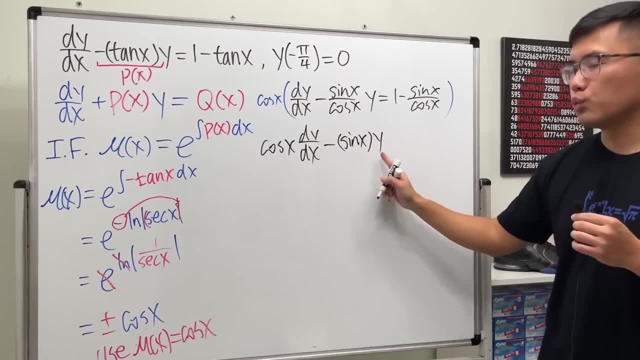 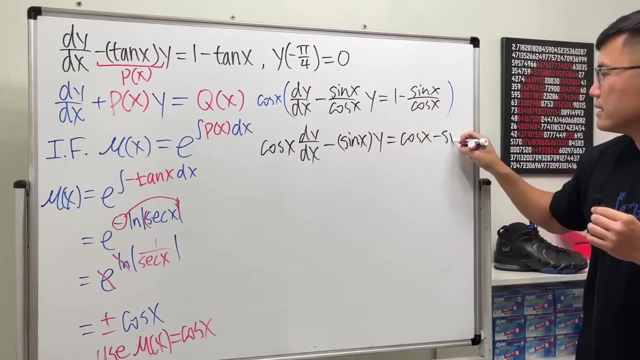 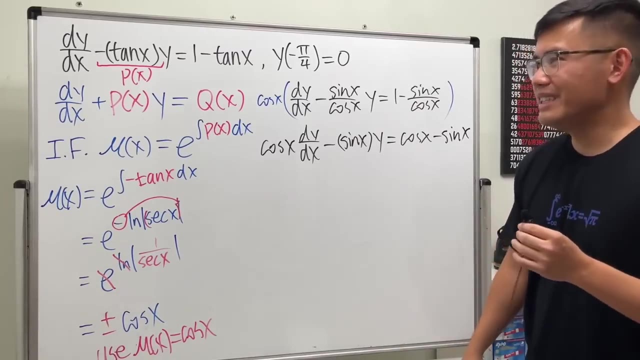 sine x times y- and let me put parentheses because y is not inside of the sign- and then cosine x here, and, lastly, we have the minus sine x. cool, and now. what, though, you know, this is so cool about the integrating factor? because the left hand side 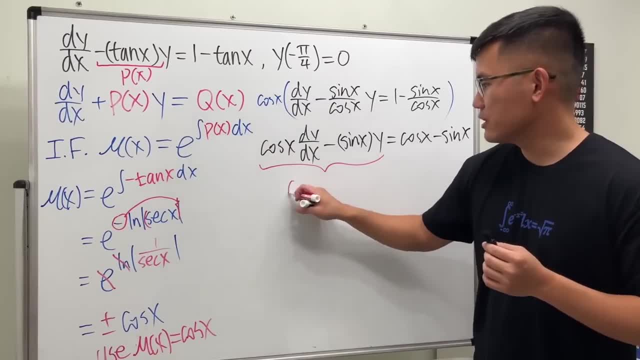 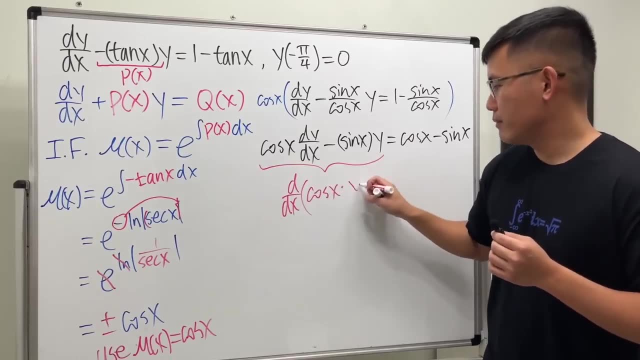 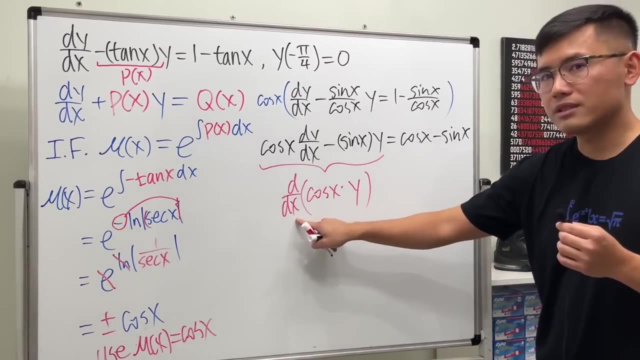 it's actually a derivative, derivative of what? check this out. it's the derivative of cosine x times y. you don't trust me? have a look. how do you differentiate cosine x times y with respect to x? y is a function of x. we will have to use the product rule. check this out first one. 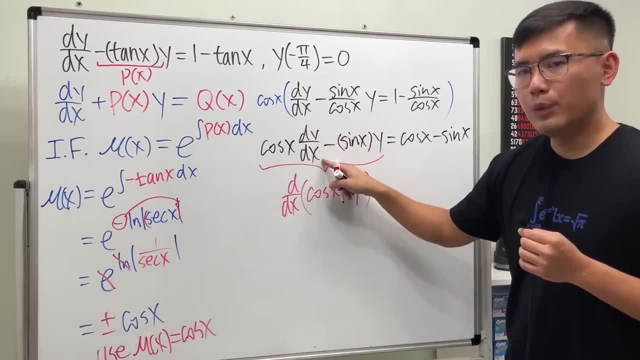 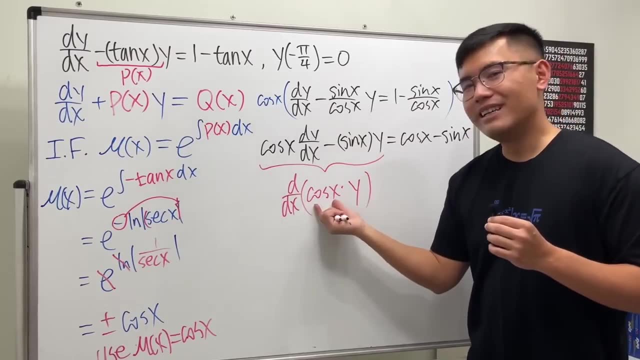 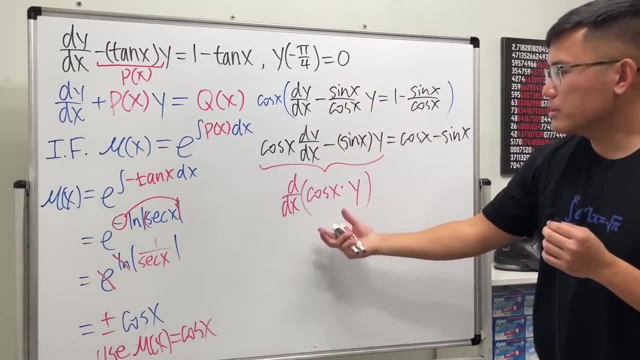 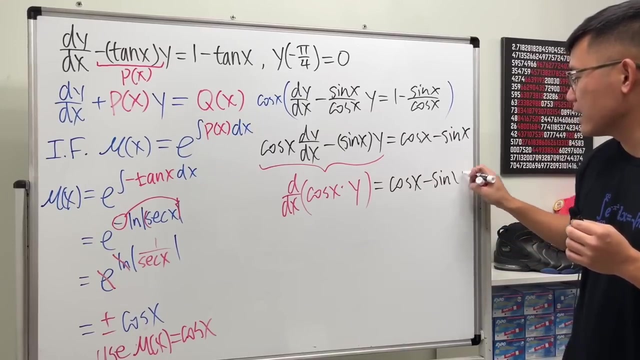 times the derivative second, namely dy, dx. and then we add: don't worry, we add the second function times. the derivative of the first derivative of cosine x is negative sine x, see, so the left hand side is actually just a derivative of cosine x times y, and then the right hand side, we have cosine x minus sine x. what do we do next, though? 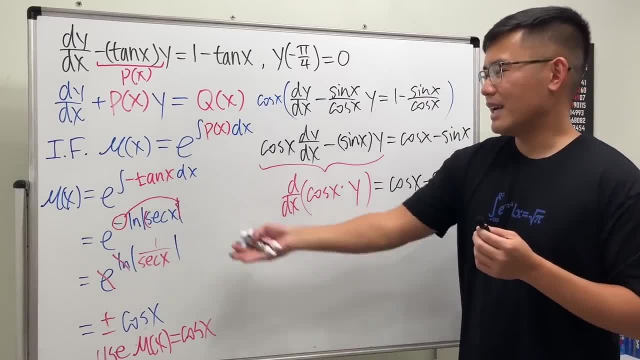 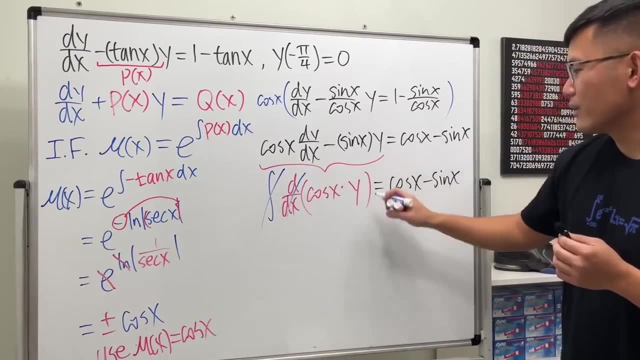 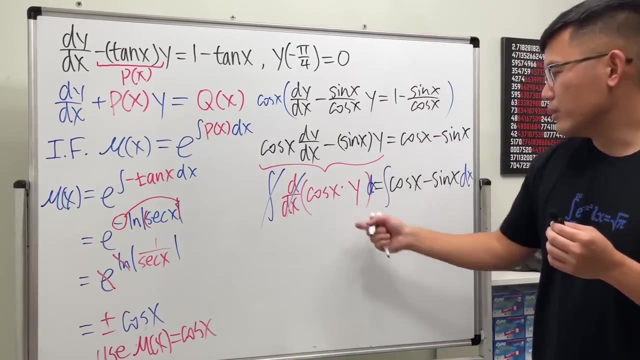 well, when we solve differential equation. yeah, even though integrated already, but let's integrate it again, because if we integrate this integral and derivative, cancel right and we'll be in the x world. so integrate both sides. on the left hand side, there's nothing to do, just write down cosine x times y and this: 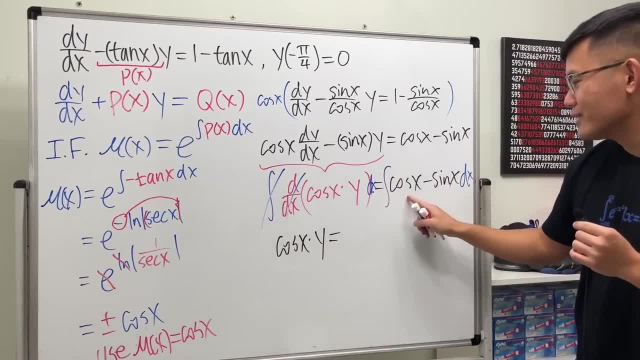 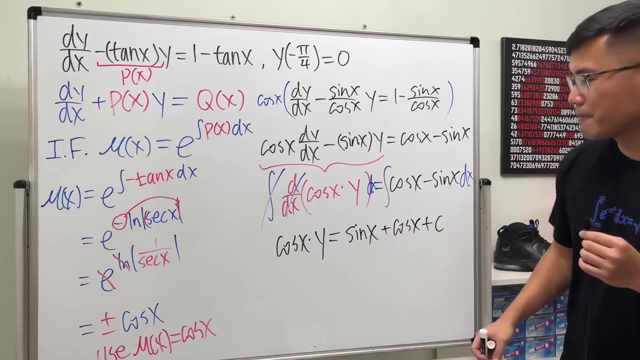 is equal to the derivative. the integral of cosine x is positive sin x and the integral of negative sine x is positive. cosine x: yeah, and then plus c, yeah. alright, now i will define everybody by cosine x, so we can get the amenity factor by×cosx.